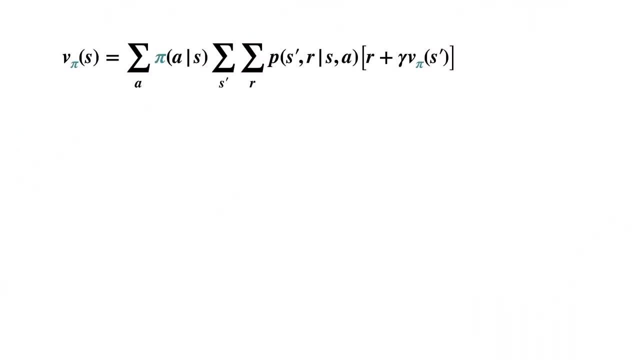 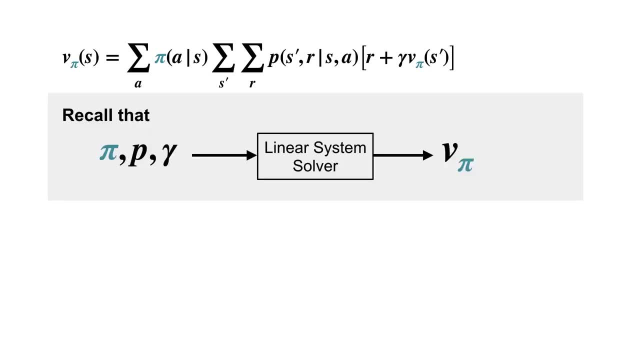 of politicians for each state. So the problem of policy evaluation reduces the solving of this system of linear equations. In principle, we could approach this task with a variety of methods, from linear algebra, In practice, the iterative solution. methods of dynamic programming are more suitable for 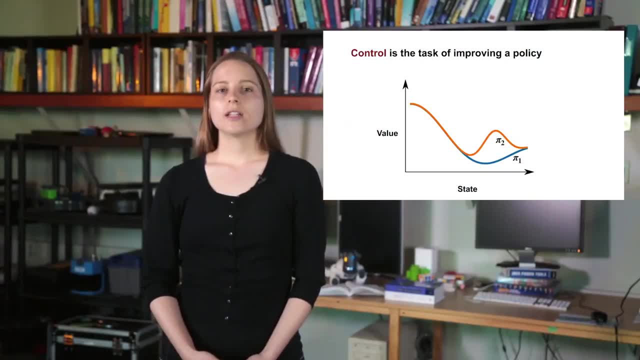 general MDPs Control is a task of improving a policy. Recall that a policy. pi is considered as good as or better than pi. the value under pi2 is greater than or equal to the value under pi1. in every state We say pi2 is strictly better than pi1 if pi2 is as good as or better than pi1. and there 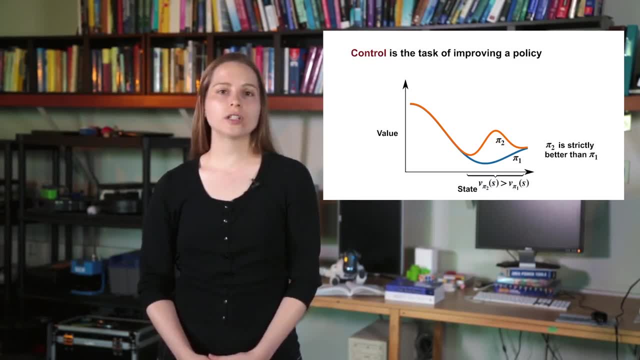 is at least one state where the value under pi2 is strictly greater than the value under pi1.. The goal of the control task is to modify a policy to produce a new one which is strictly better. Moreover, we can try to improve the policy repeatedly to obtain a sequence of better. 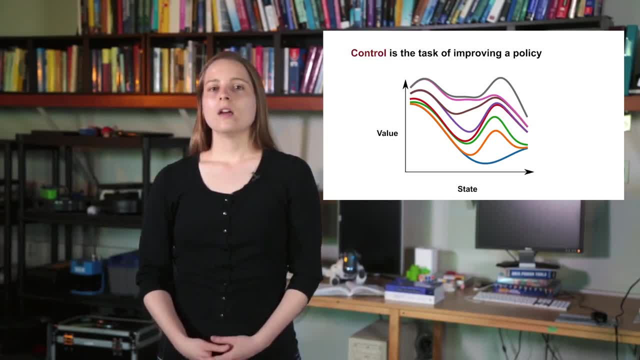 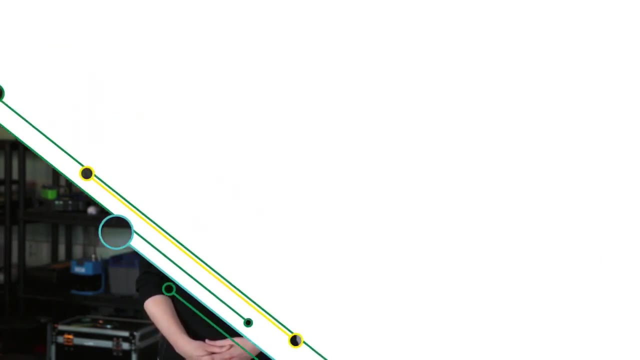 and better policies When this is no longer possible. it means there is no policy which is strictly better than the current policy, And so the current policy must be equal to an optimal policy and we can consider the control task complete. Imagine we had access to the dynamics of the environment. P. 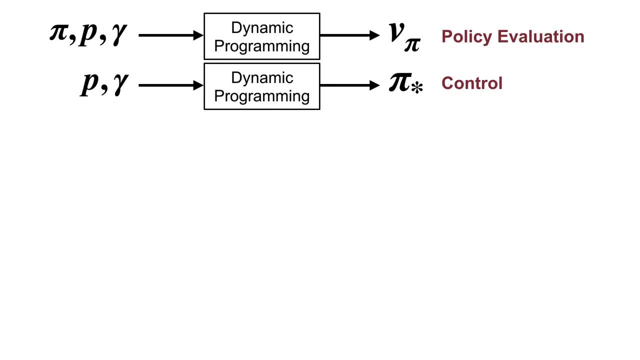 This week is all about the dynamics of the environment. Let's talk about how we can use this knowledge to solve the tasks of policy evaluation and control. Even with access to these dynamics, we'll need careful thought and clever algorithms to compute value functions and optimal policies. 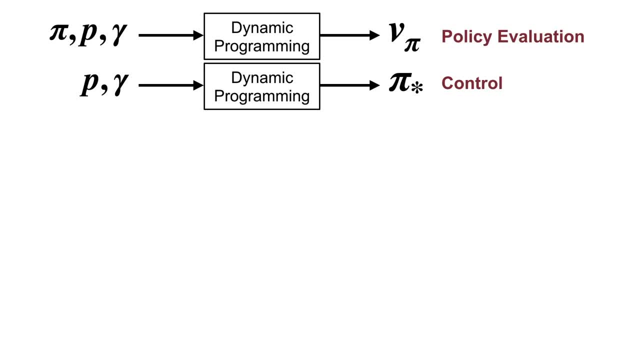 For the next several videos, we will investigate a class of solution methods called dynamic programming. for this purpose, Dynamic programming uses the various Bauman equations we've seen, along with knowledge of P, to work out value functions and optimal policies. Classical dynamic programming does not involve interaction with the environment at all.